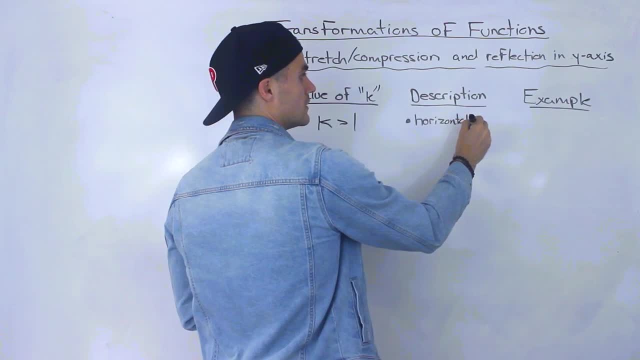 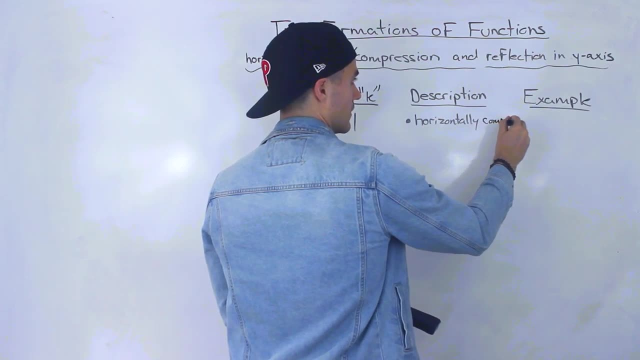 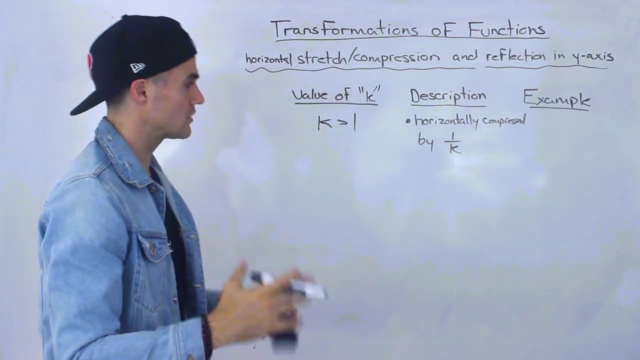 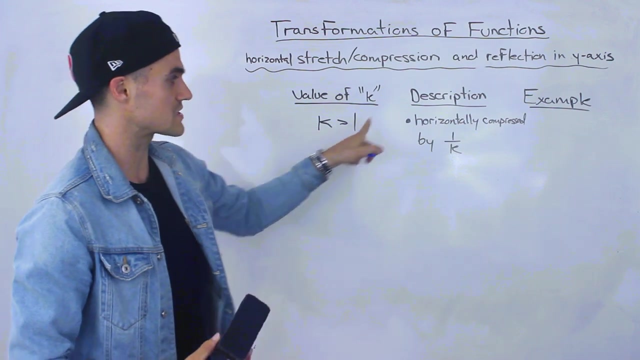 the function is horizontally- sorry, horizontally- compressed by one over k, by a factor of one over k. So here's where this is a little bit more weird compared to the a values, because you actually, when you're describing it, you have to take the 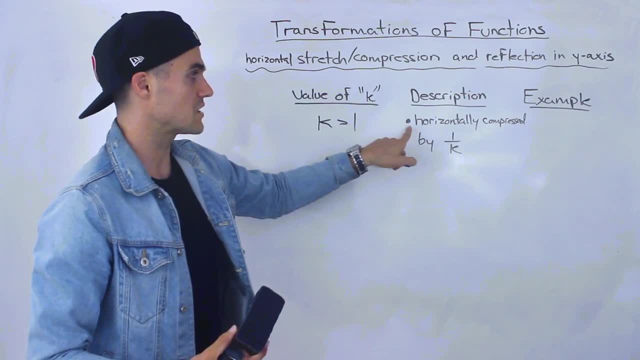 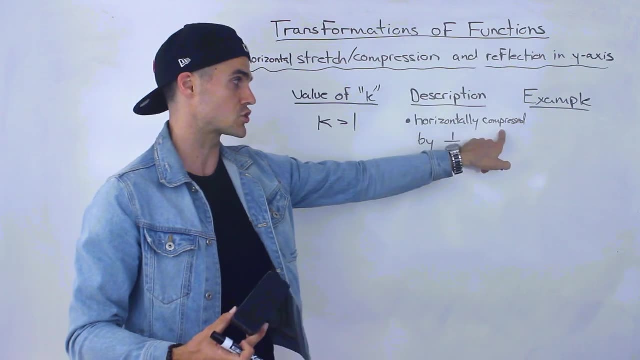 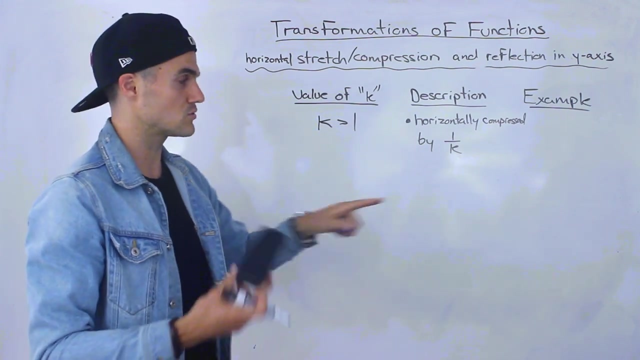 reciprocal of that value, right? So it's going to be horizontally compressed by one over k. Remember, when a was greater than one, it was vertically stretched by a, But if k is greater than one, it's horizontally compressed by one over k, right? So just be aware of the difference. 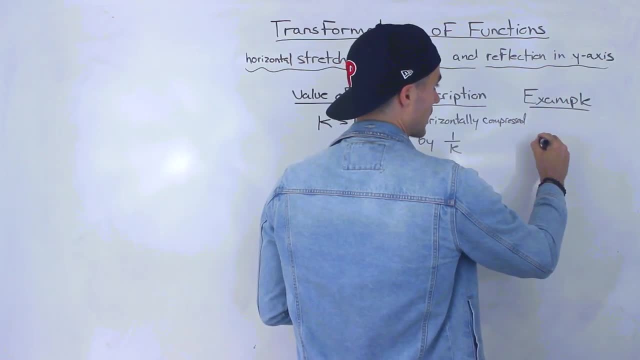 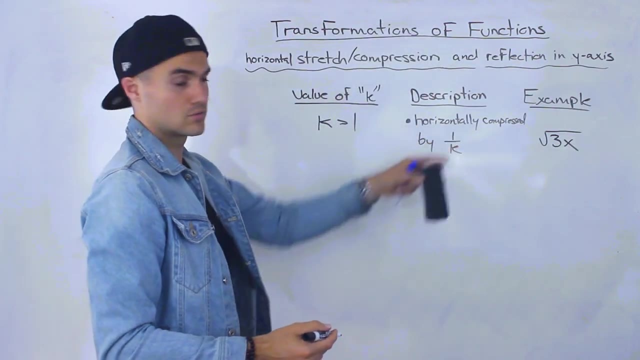 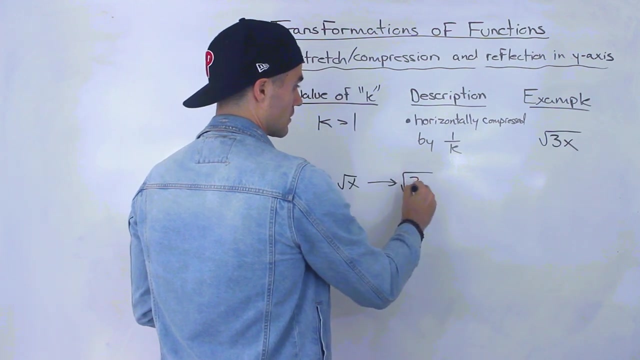 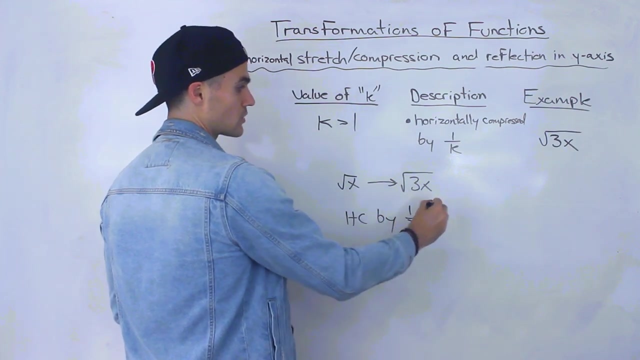 And an example of that is: let's say that we would have the square root of three, x. So notice that the k value is three. So we would say that this function, if it goes to here, it is horizontally compressed by a factor of one over three. Notice how the k value is three. 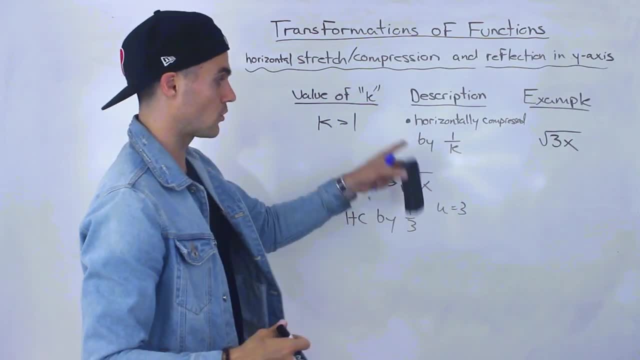 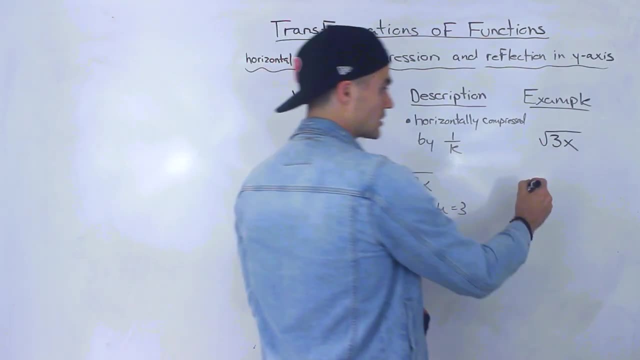 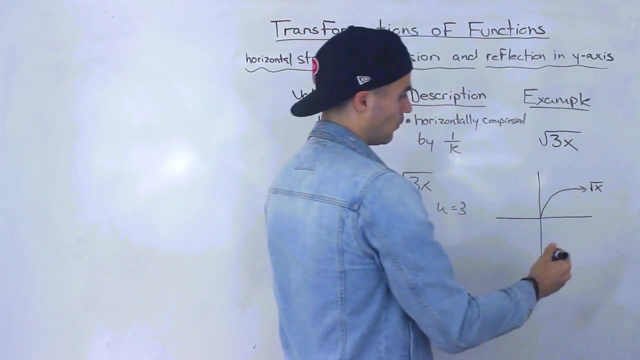 So when we describe the, the compression, the horizontal compression, we flip that three and say it's one over three. Okay, and the way that this looks compared to the square root of x- remember the square root of x- it looks like this: Well, what we would do is we would take this and horizontally compress it. 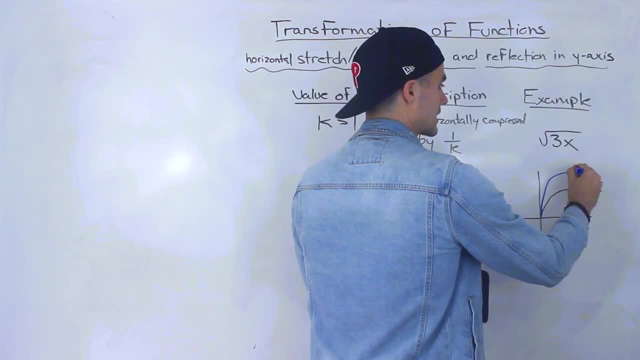 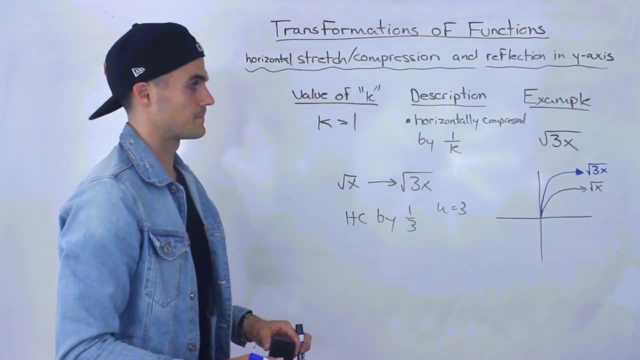 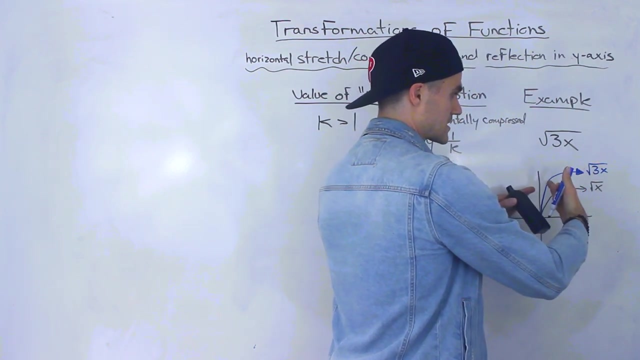 And so the way it would end up looking is like that. So this would be an example of the square root of three, x. Okay, so we're taking one more time this function, the square root of x, and horizontally compressing it by a factor of one over three, And so it ends up looking like that: 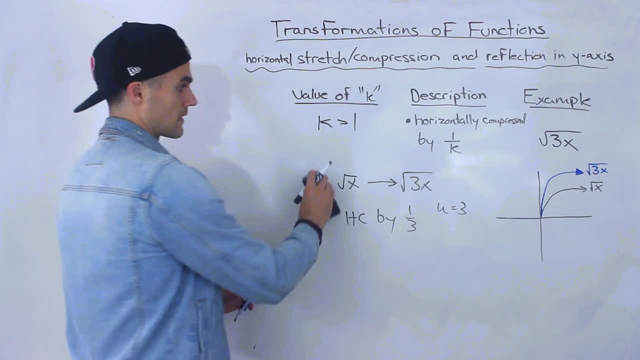 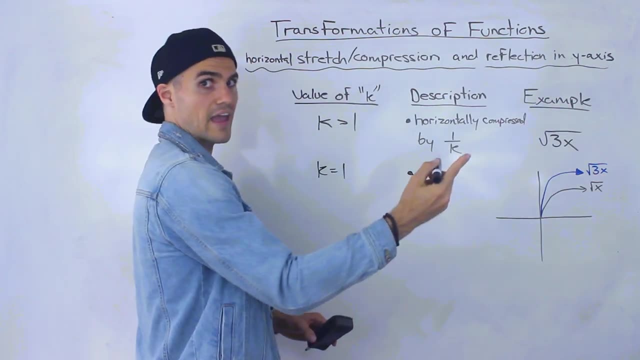 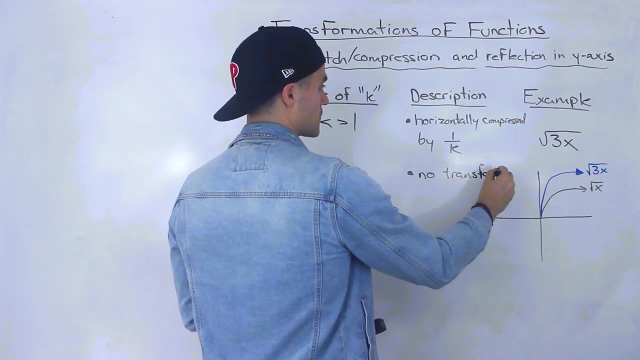 Okay, so that is the the first case. Now, if k is equal to one, then, like the a value, when the a value is equal to one, there's not going to be any transformation, Because we would still have just the square root of x, right, There would be like a one over here. 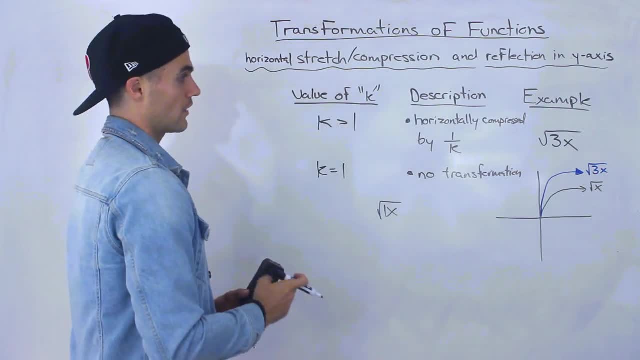 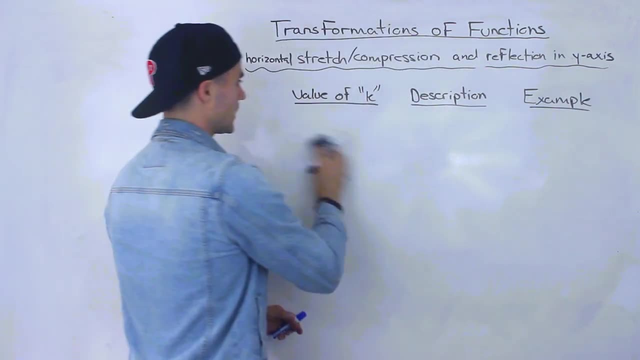 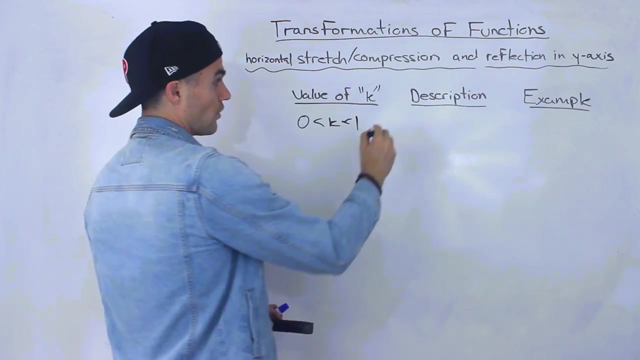 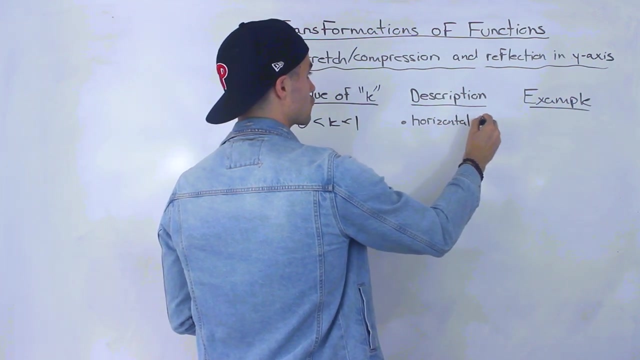 so it does not change. So if k is one, there is no transformation. Now, what if k is between zero and one? What's going to happen then? Well then, we would say there is a horizontal stretch by a factor, by the reciprocal. 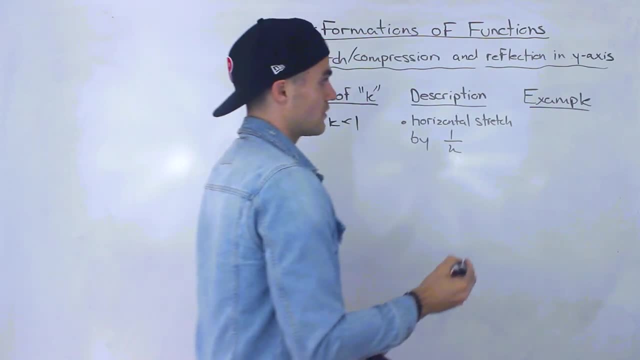 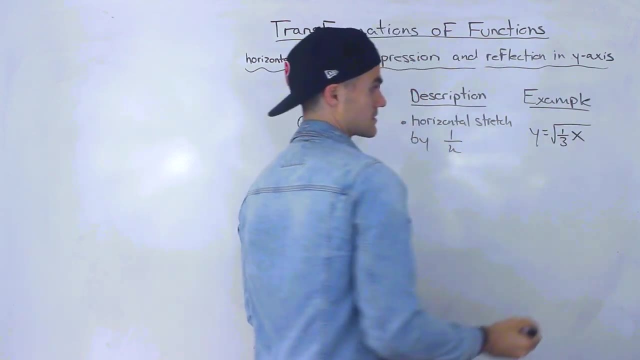 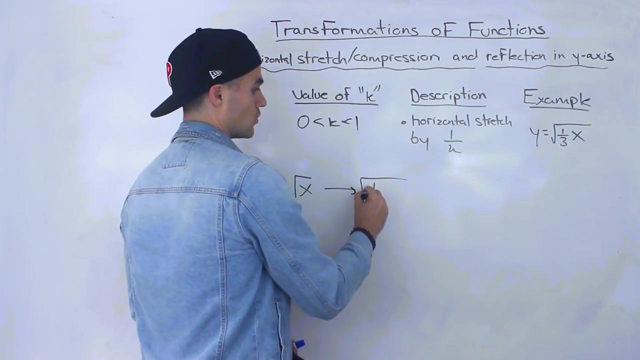 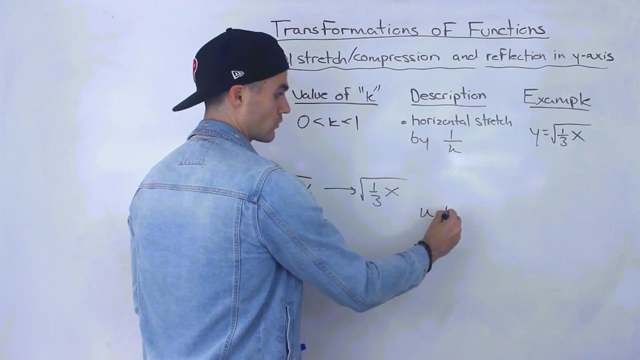 And then again there's also a three- passé situation in which k outside yed um. so the approach is that we would say, particularly to problems which we would look at later, that k outside x were going to be a complex situation, again by one over k. Okay, so an example of this is: if we have, y is equal to the square root of one over three x. 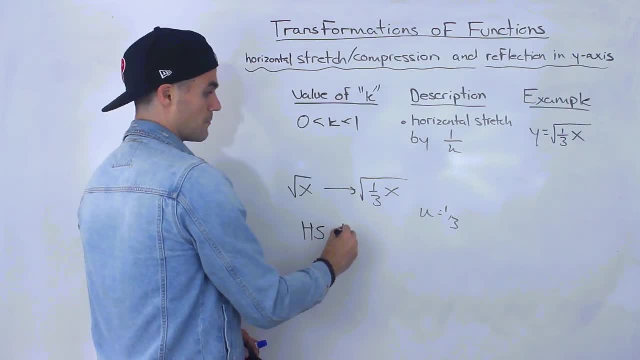 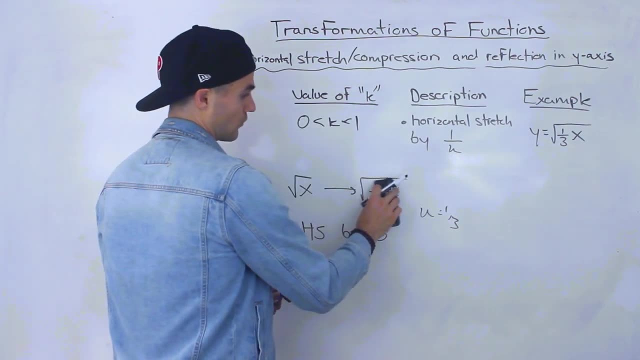 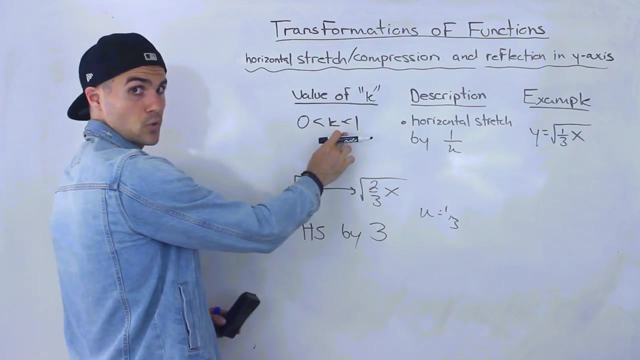 case. so we would say there's a horizontal stretch by the reciprocal of this, so we would say by 3, okay, And you've got to also look out for other fractions, like let's say this was 2 over 3, notice, 2 over 3 is between 0 and 1, so the k-value would be 2 over 3, so we would 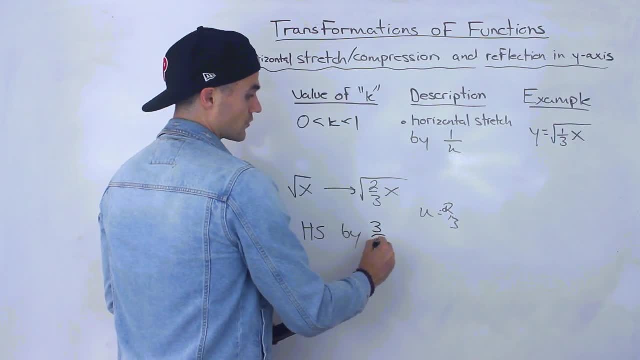 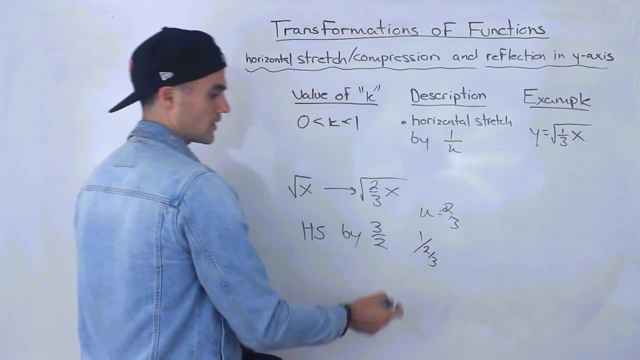 say that there's a horizontal stretch by 3 over 2,, which is the reciprocal of 2 over 3, so it would be like 1 over 2 over 3,, which ends up being 3 over 2, alright. 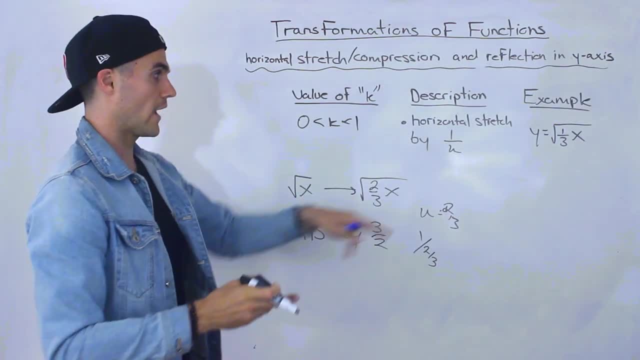 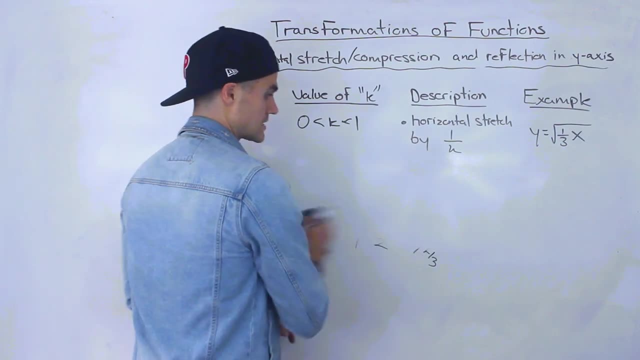 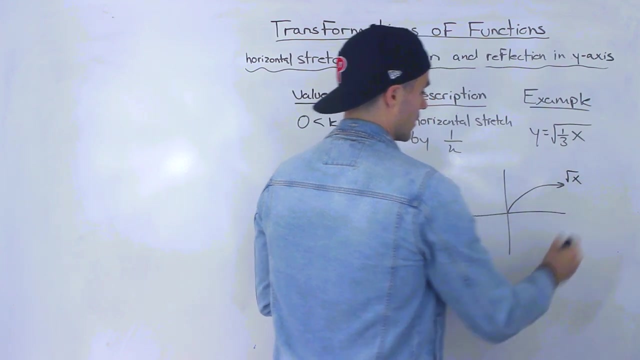 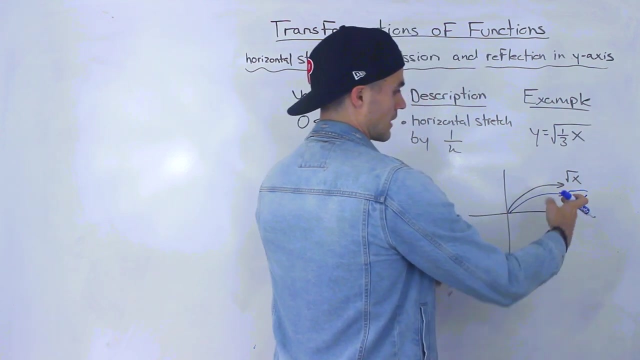 So just remember the k-value, whatever it is. you're flipping it when you are describing the transformation. okay, And the way that this is going to look graphically if we graph these squares: okay, Square root of x here. well, the square root of 1 over 3x is going to look like this: okay, 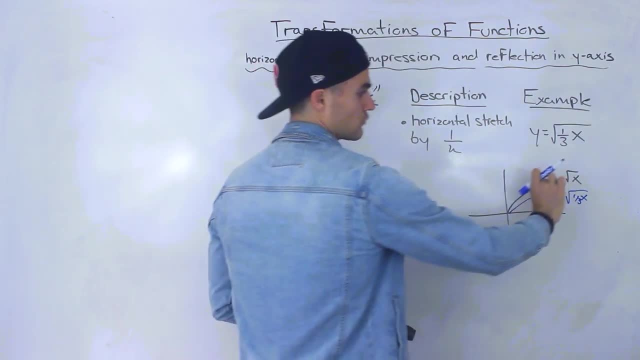 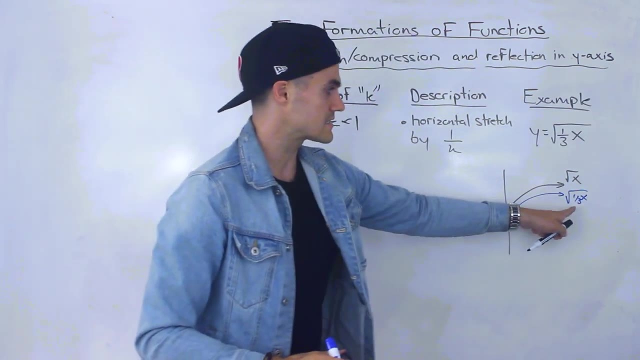 It's horizontally stretched by a factor of 3, so if we take this and we horizontally stretch it, we would end up getting this over here, alright. So that's how the square root of 1 over 3x looks like compared to the square root of. 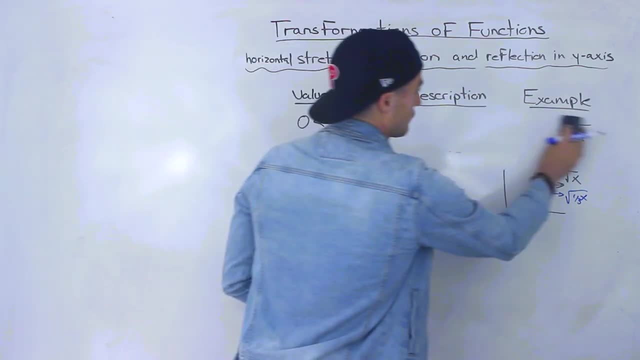 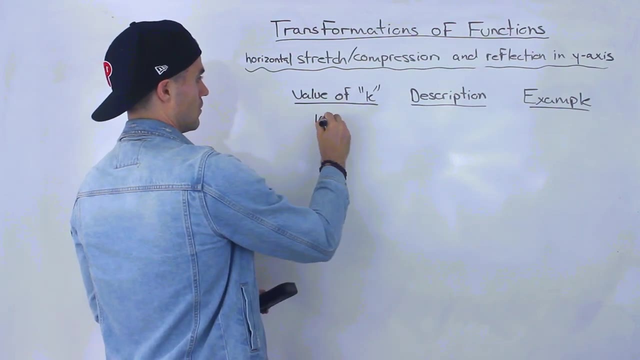 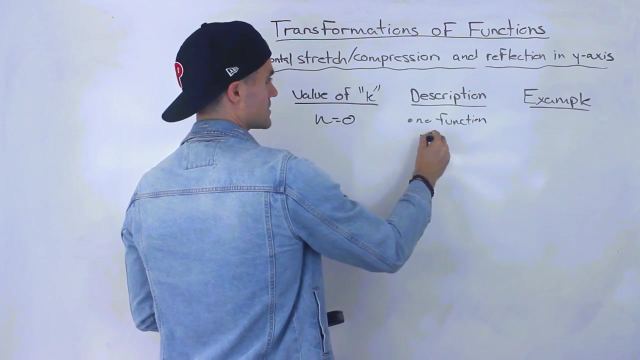 x. alright. Now what if k is equal to 2, over 2?? If k is equal to 0,? well, if k is equal to 0, then there's no function. You'll end up just having: y is equal to 0, right, because we'll have the square root. 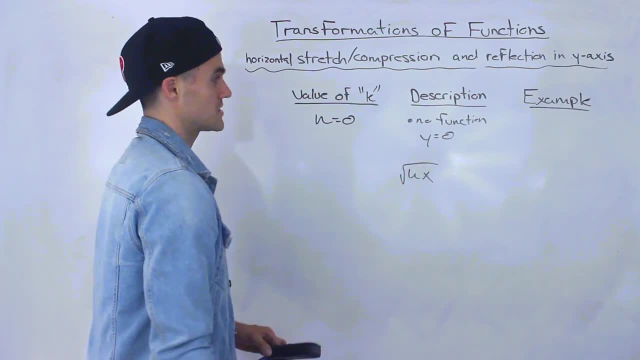 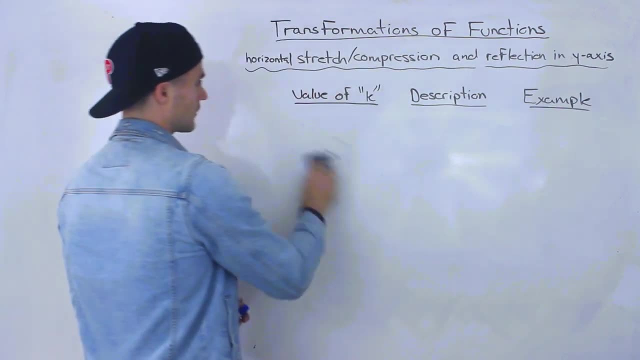 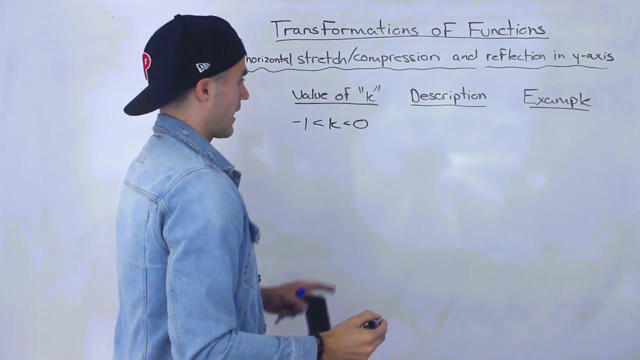 of kx. k is 0, this whole thing is going to be 0, right, So you most likely won't run into a scenario like that. The next case is if k is between negative and positive, Negative 1 and 0. 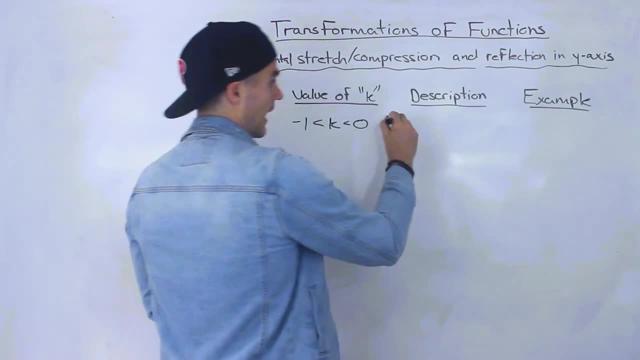 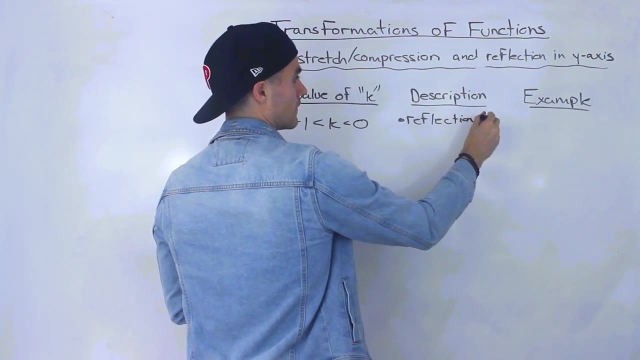 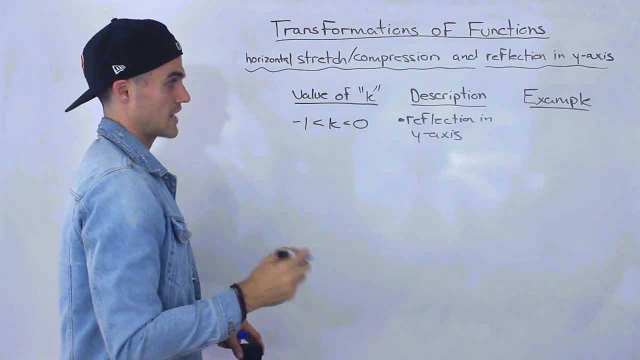 So notice, in this case k is going to be negative for sure, and whenever k is negative, then there's a reflection in the y-axis. okay, So a reflection in the y-axis is for sure going to happen if the k value is negative. 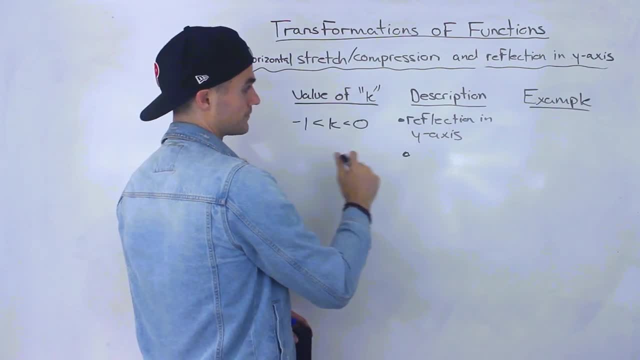 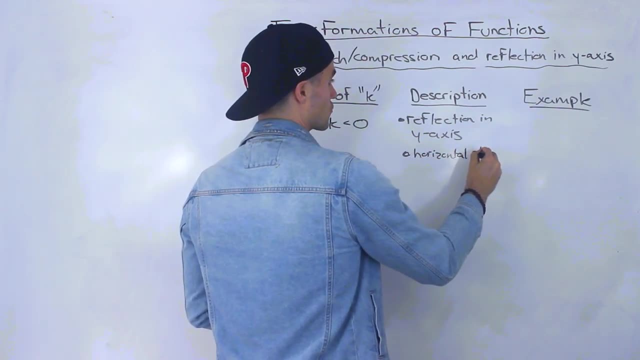 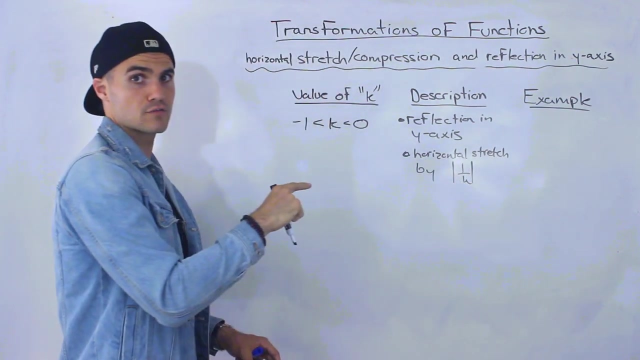 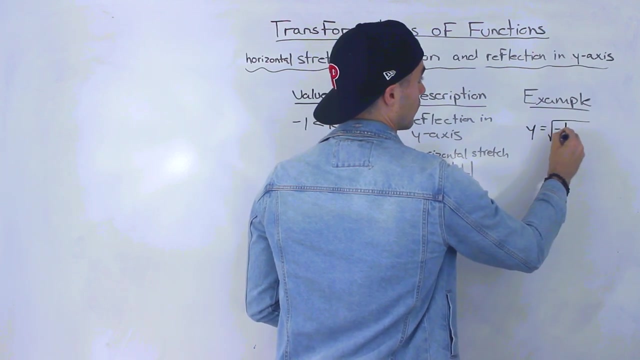 and in this specific case, if it's between 0 and negative 1, then we would say there is a horizontal stretch by the absolute value of 1 over k. We would just say the positive, like we did with the a. So, for example, if we had, y equals the square root of negative 1 over 3x. 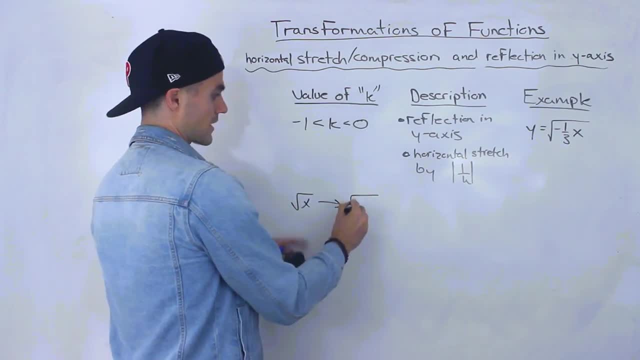 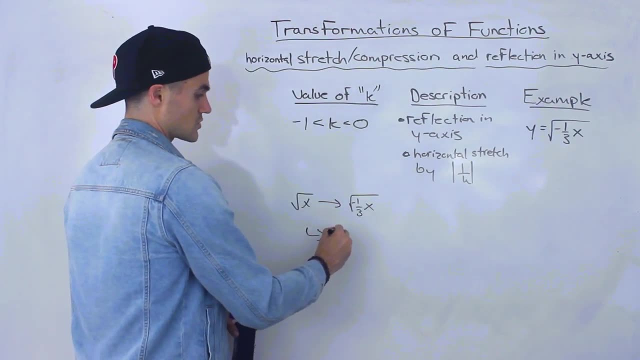 So let's do this here. We're taking square root of x, we're transforming it to the square root of negative 1 over 3x. Well, if we describe these transformations, we would say: there's a reflection in the y-axis. 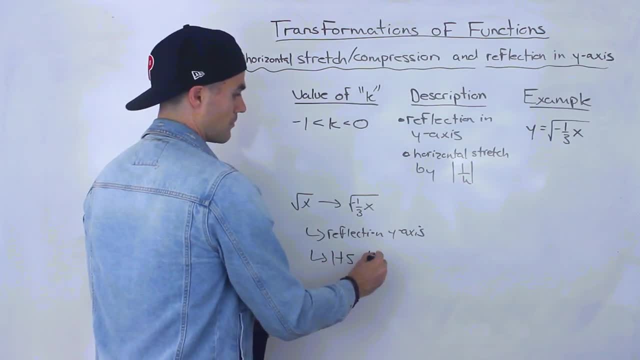 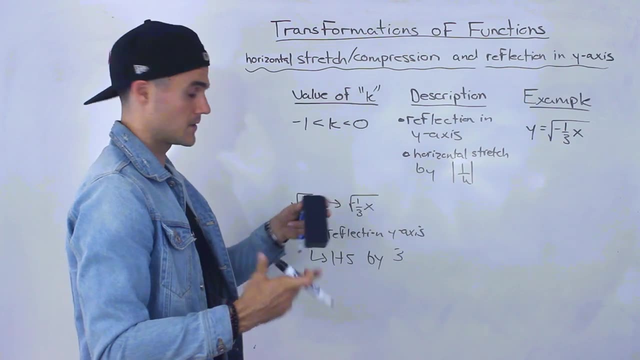 and then we would say there's a horizontal stretch by 3, by the reciprocal of the absolute value. The absolute value of negative 1 over 3 is 1 over 3, and then the reciprocal of it is just 3, right. 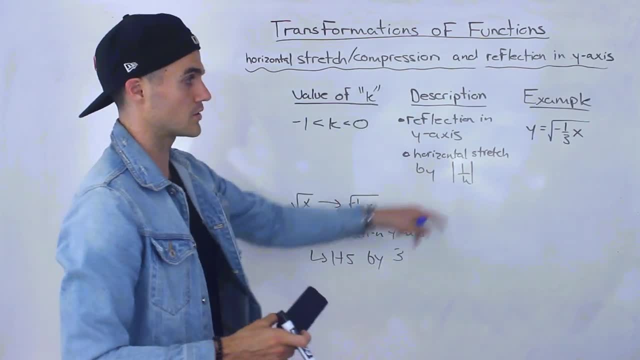 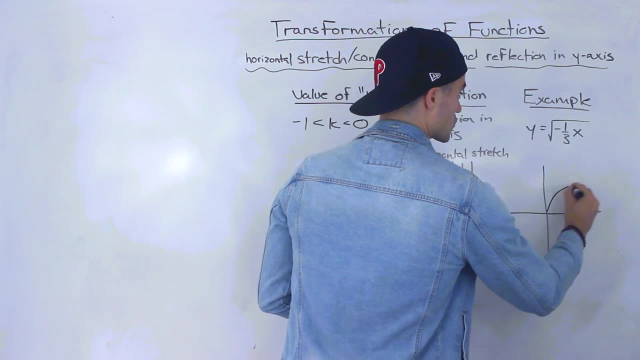 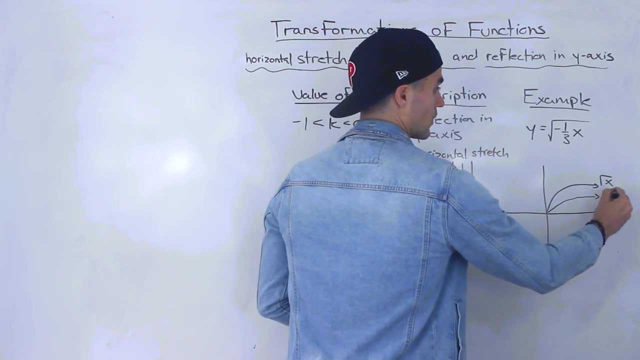 So, whatever that k value is, remember you're always just flipping it when you are describing the transformation And the way that this is going to look compared to the square root of x. So this is the square root of x. We mentioned that this is the square root of 1 over 3x.